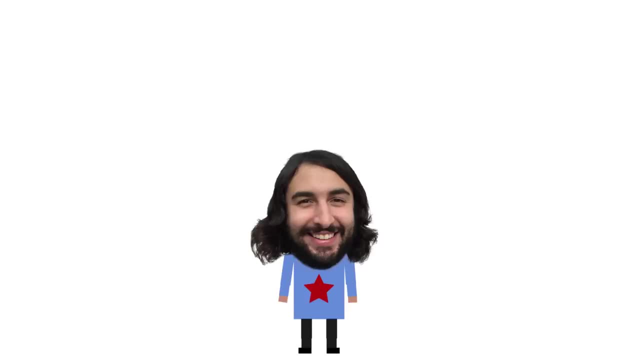 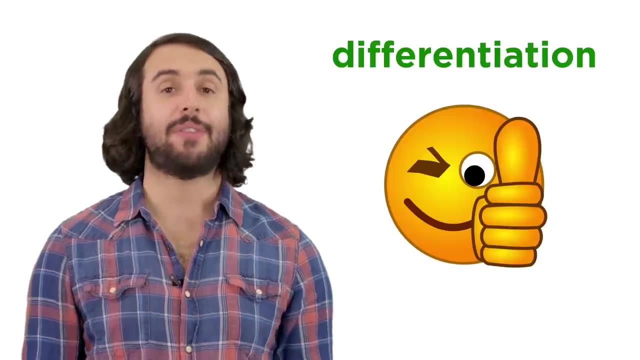 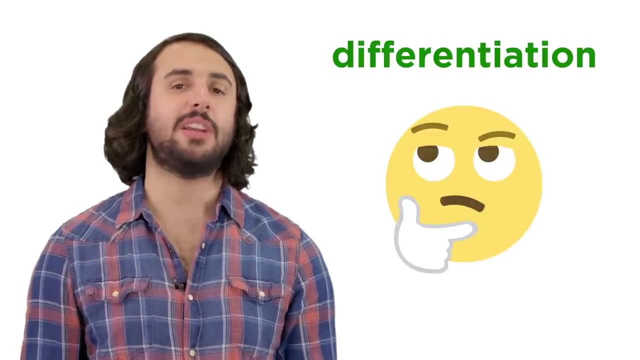 It's Professor Dave. let's find maxima and minima. By now we have a solid concept of differentiation, what it is and how to do it with a variety of functions. So let's continue to learn about some applications for differentiation. 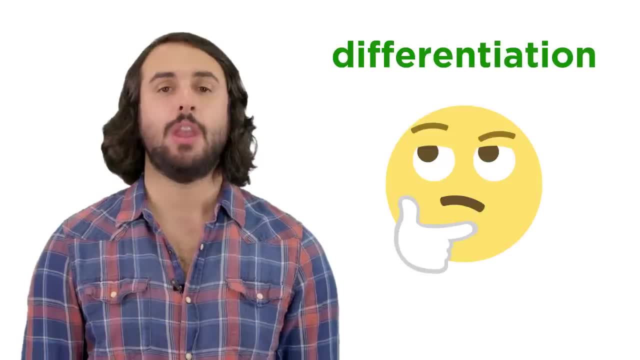 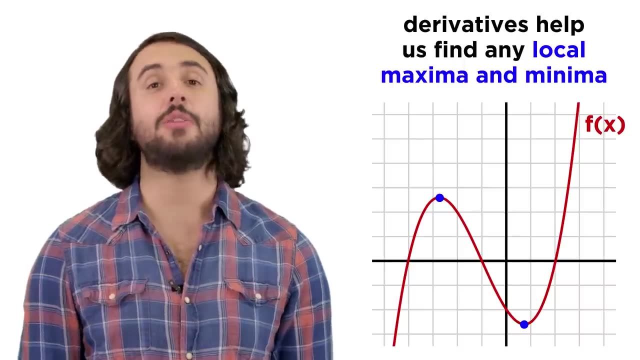 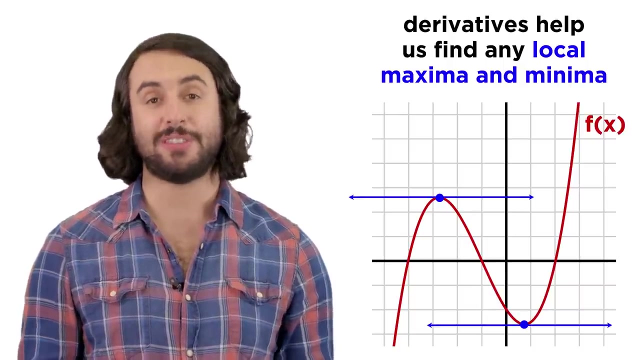 How is it useful and what can it tell us about a function? Well, if a function looks like this, with local maxima and minima, then a derivative can be very useful in figuring out where those are exactly. Let's recall that if a derivative can be interpreted as the slope of a tangent line, 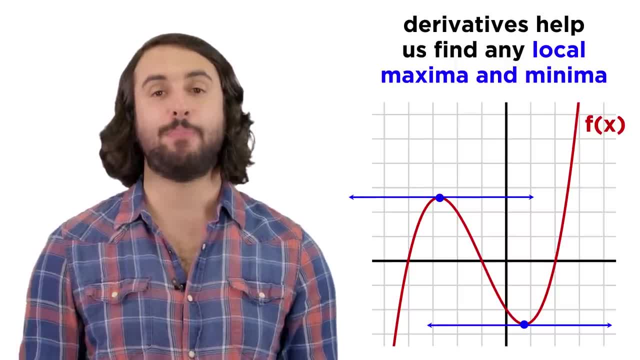 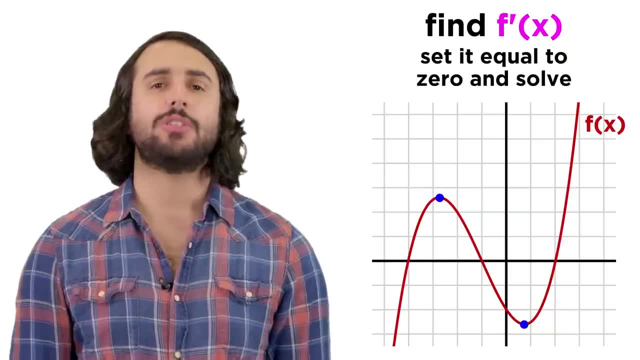 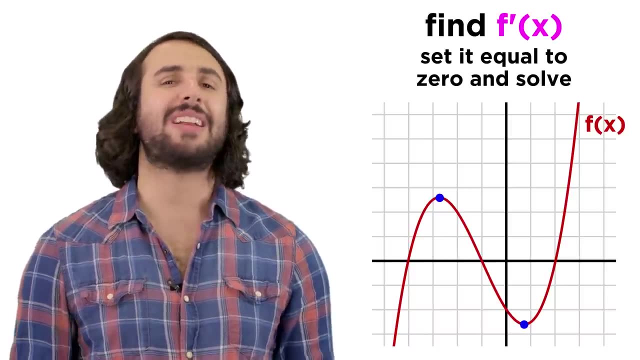 and the tangent line at any maximum or minimum must be perfectly horizontal, then the derivative of a function at any of these points must equal zero. So to find them, all we need to do is take the derivative and find the zero. There are countless applications for this, and we will go over many of them a little. 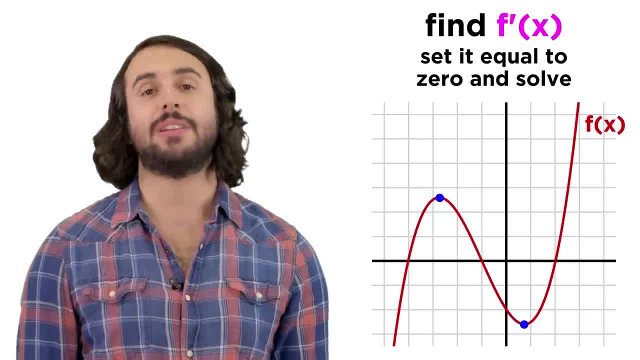 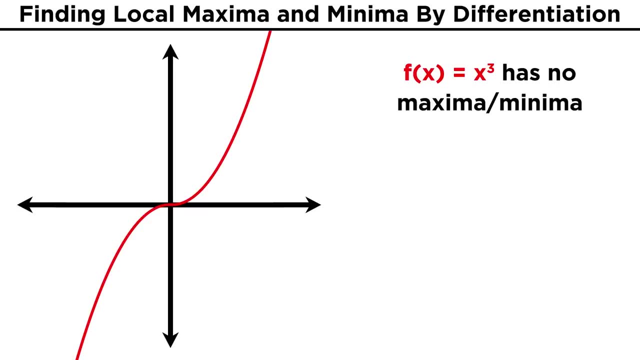 later, when we look at optimization problems. For now, let's not worry about application, let's just get some practice in finding these values. Of course, some functions have no maxima or minima. Take x cubed, for example. This function is constantly increasing as we move left to right, from negative infinity. 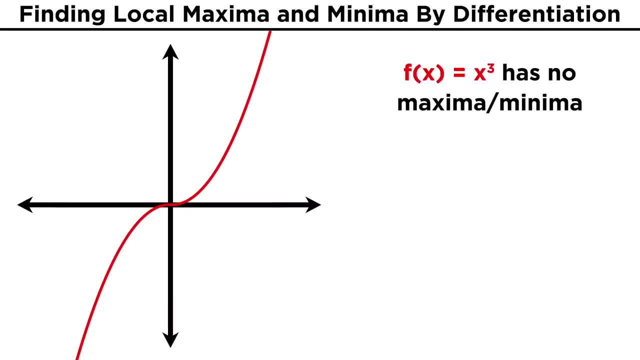 to positive infinity. So there are no maxima or minima to speak of. Some functions have absolute maxima and minima. This would be something like sine of x. This function will never be greater than one, which is its value at any input. that is half. 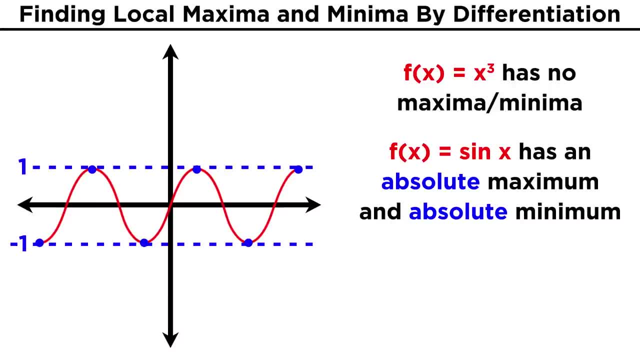 pi, plus or minus any multiple of two pi. Likewise, it will never be less than negative one, which is its value at any of these inputs. So these are absolute maxima and minima. If we zoom in on a specific function, we can see that it is always greater than one. 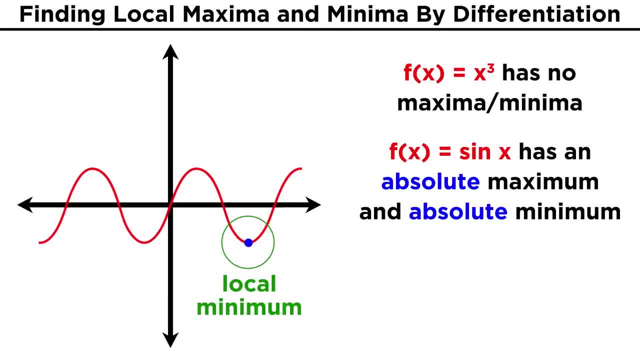 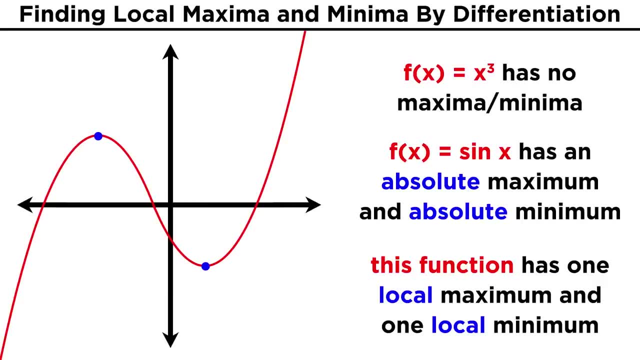 If we zoom in on a specific portion, we can identify a local or relative maximum or minimum, but this will repeat in either direction. Some functions instead will have a finite number of local maxima or minima. This is just the highest or lowest point on the curve in a particular section which we 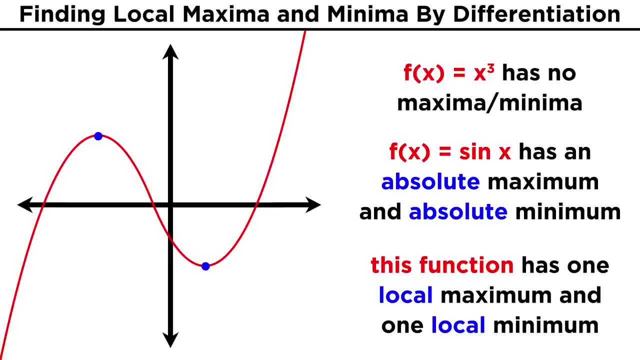 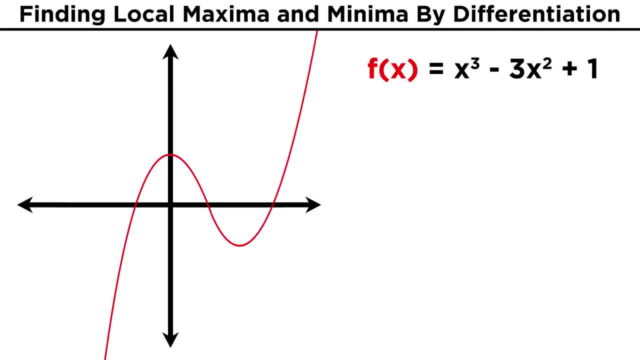 can identify as any point where the function changes direction. Let's look at the function x cubed minus three pi. Let's look at the function x cubed minus three pi. Let's look at the function x squared minus three. x squared plus one. 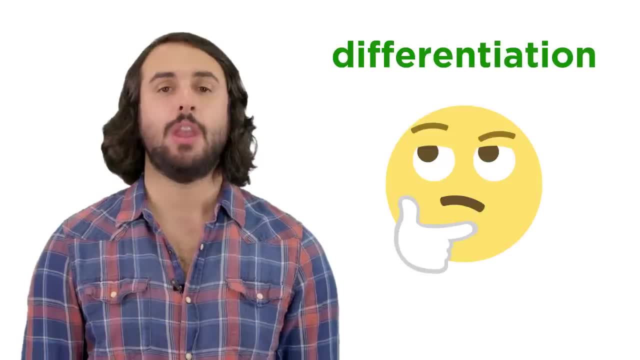 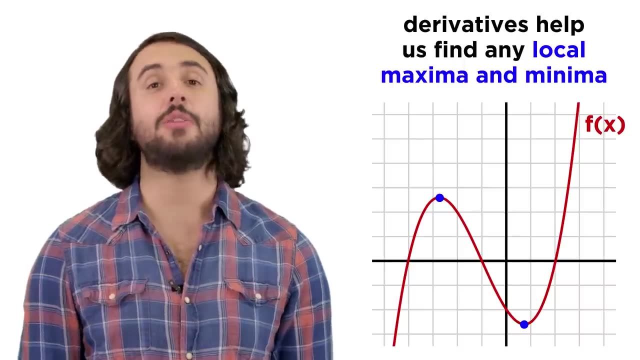 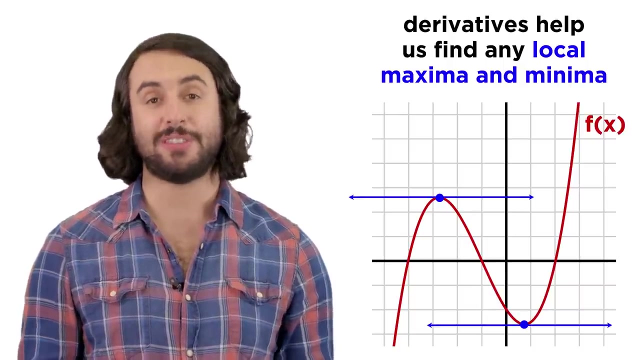 How is it useful and what can it tell us about a function? Well, if a function looks like this, with local maxima and minima, then a derivative can be very useful in figuring out where those are exactly. Let's recall that if a derivative can be interpreted as the slope of a tangent line, 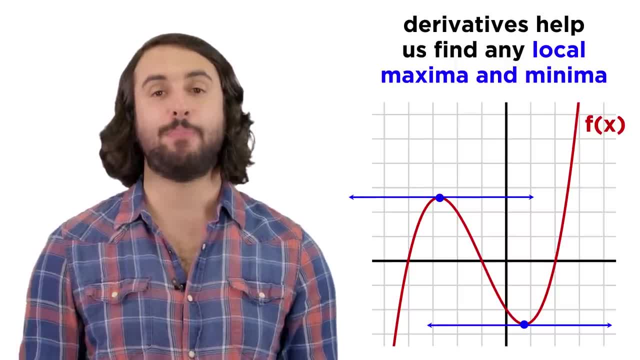 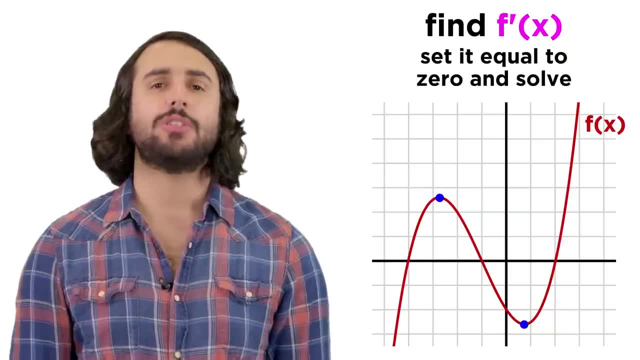 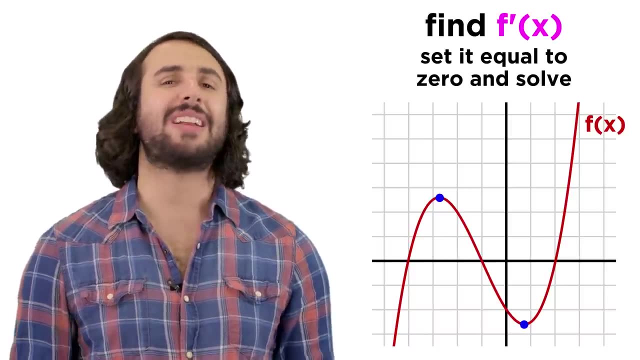 and the tangent line at any maximum or minimum must be perfectly horizontal, then the derivative of a function at any of these points must equal zero. So to find them, all we need to do is take the derivative and find the zero. There are countless applications for this, and we will go over many of them a little. 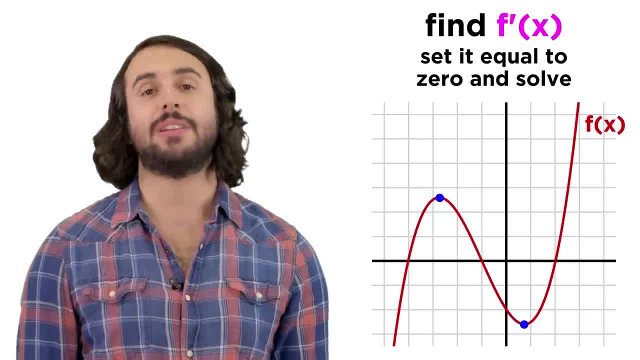 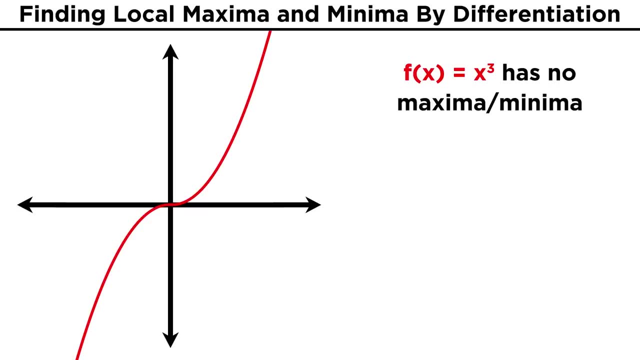 later, when we look at optimization problems. For now, let's not worry about application, let's just get some practice in finding these values. Of course, some functions have no maxima or minima. Take x cubed, for example. This function is constantly increasing as we move left to right, from negative infinity. 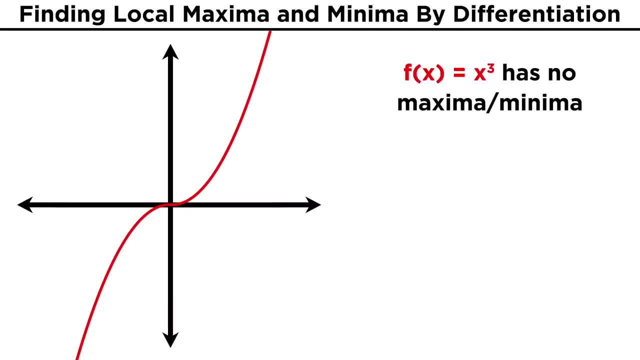 to positive infinity. So there are no maxima or minima to speak of. Some functions have absolute maxima and minima. This would be something like sine of x. This function will never be greater than one, which is its value at any input. that is half. 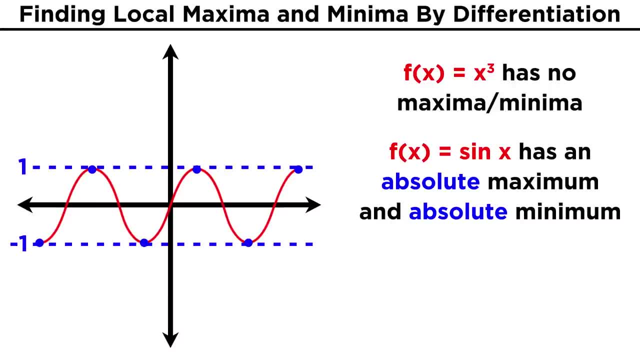 pi, plus or minus any multiple of two pi. Likewise, it will never be less than negative one, which is its value at any of these inputs. So these are absolute maxima and minima. If we zoom in on a specific function, we can see that it is always greater than one. 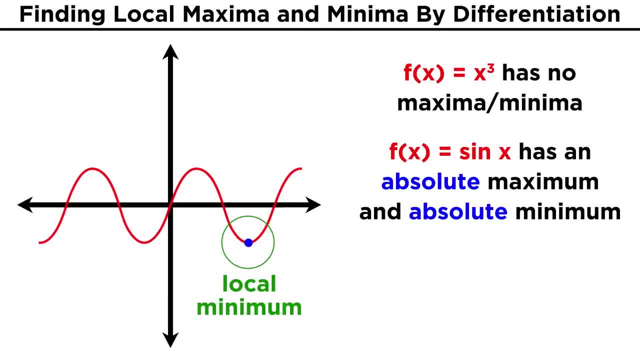 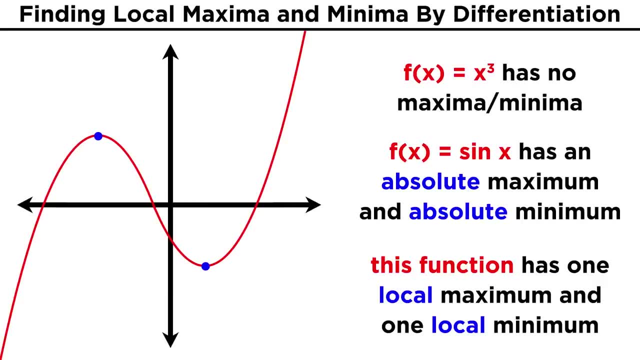 If we zoom in on a specific portion, we can identify a local or relative maximum or minimum, but this will repeat in either direction. Some functions instead will have a finite number of local maxima or minima. This is just the highest or lowest point on the curve in a particular section which we 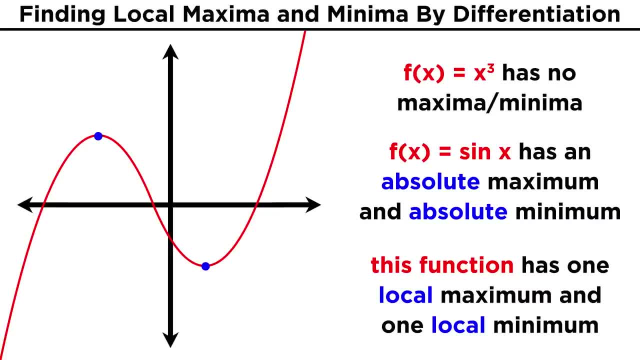 can identify as any point where the function changes direction. Let's look at the function x cubed minus three pi. This function is always greater than one. If we zoom in on a specific function, we can see that it is always greater than or minus. 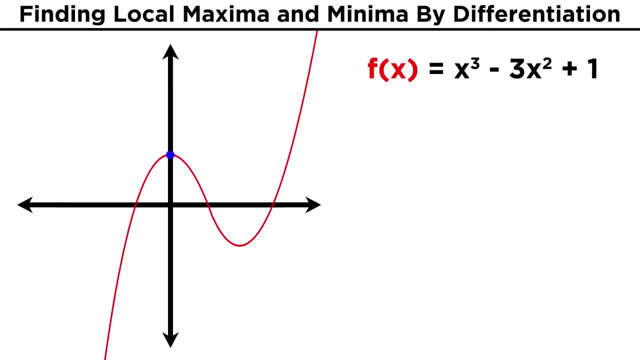 three x squared plus one. There is one local maximum and one local minimum. Where do these occur? Well, as we said, let's take the derivative. That will be three x squared minus six x. We can factor out a three x from both terms to get three x times x minus two. 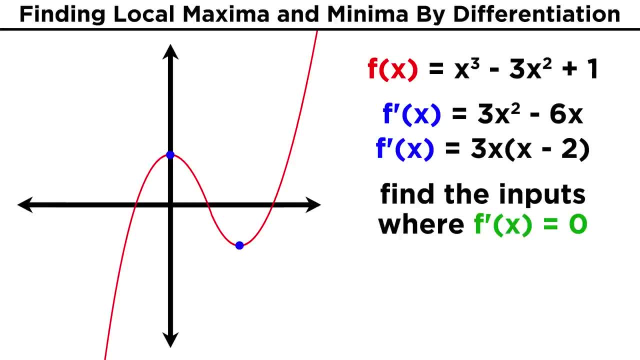 Now we want to find the input values for which this derivative equals zero, because those will be the points on the x-axis. Let's run the function with horizontal tangent lines. Well, this is just basic algebra. If x is zero, f prime is zero. 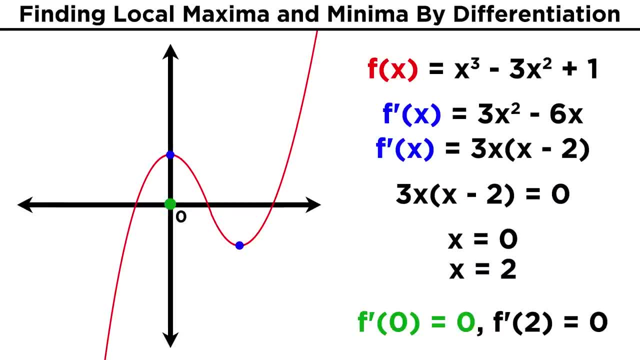 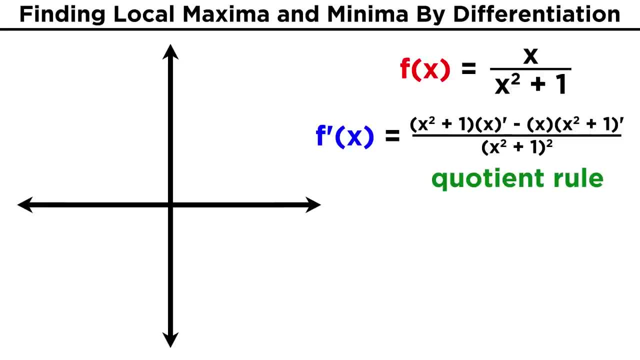 What about x over the quantity of x? Again, we must take the derivative, and for that we need the quotient rule. Remember it's bottom times, the derivative of the top minus top times the derivative of the bottom over bottom squared. 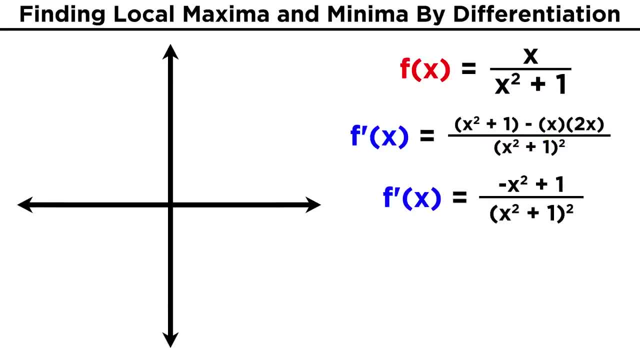 Here. that gives us this, and we can simplify to get negative x squared plus one on top. Now remember to find the zeros of a rational function like this one. we need to find the one. we just need to find the zeros of the numerator, since zero over anything is zero. 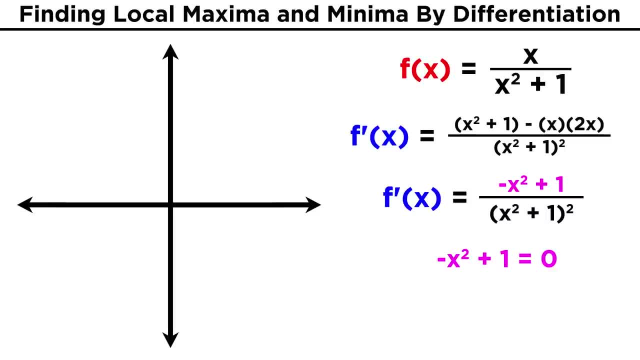 So let's set negative x squared plus one equal to zero. We rearrange to get x squared equals one. take the square root of both sides and x must be equal to plus or minus one. That means that x equals negative one and one will give local maxima or minima on the 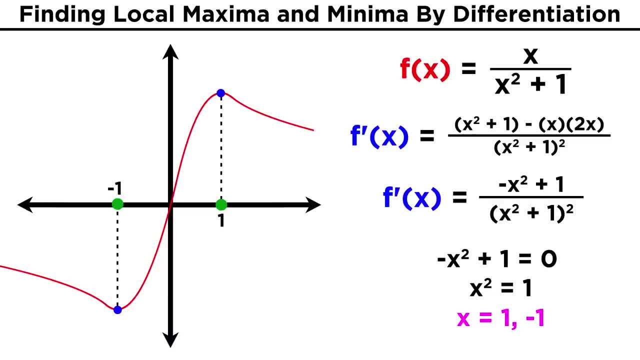 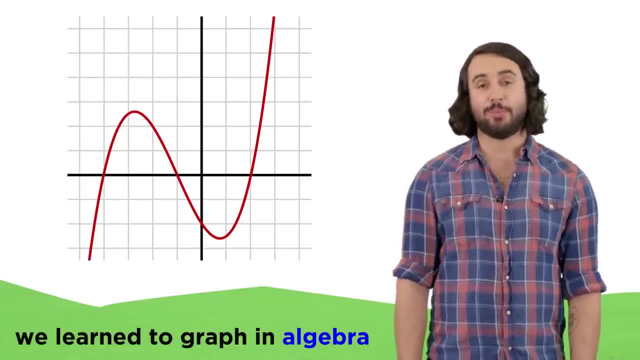 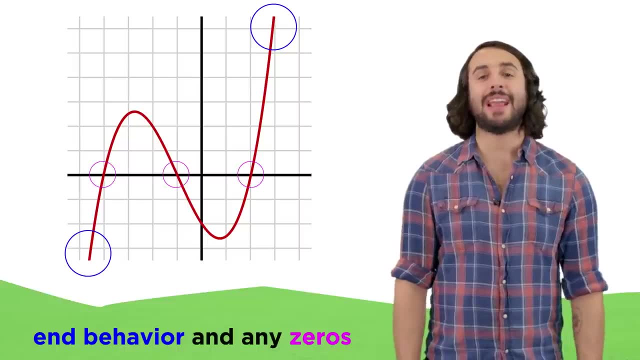 function, and in fact the function looks like this. So this is one great application of differentiation. In algebra we learned how to get a rough sketch of a higher degree polynomial by finding the end behavior and its zeros, but it was always a pretty rough sketch, as we never 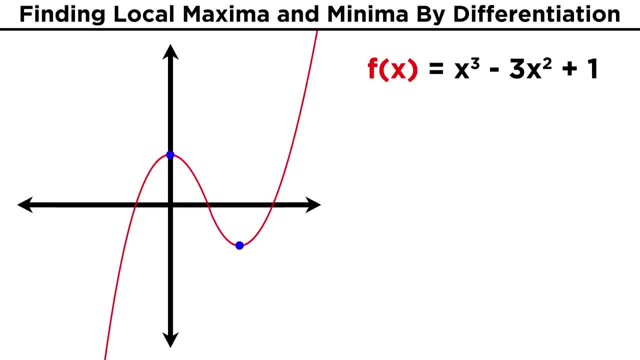 There is one local maximum and one local minimum. Where do these occur? Well, as we said, let's take the derivative. That will be three x squared minus six x. We can factor out a three x from both terms to get three x times x minus two. 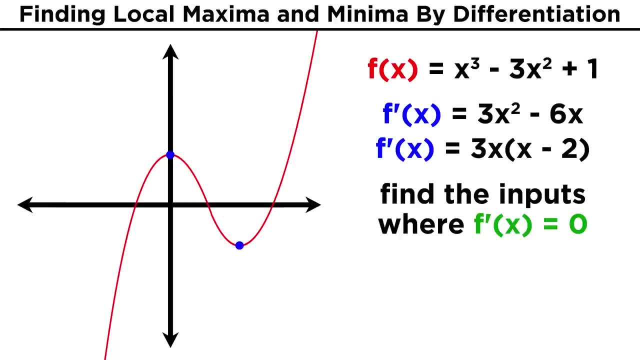 Now we want to find the input values for which this derivative equals zero, because those will be the points on the x-axis. How do we find the function with horizontal tangent lines? Well, this is just basic algebra. If x is zero, f prime is zero. 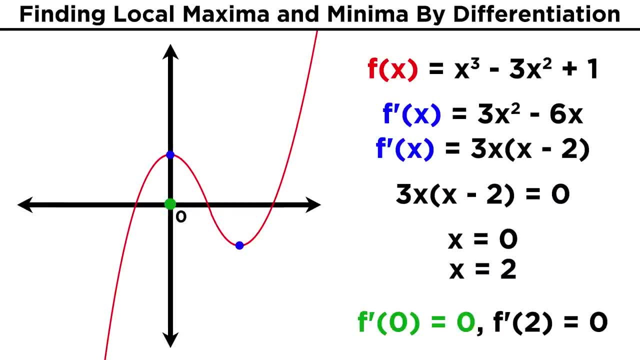 If x is two, f prime is zero. So the local maximum occurs at x equals zero and the local minimum occurs at x equals two. Of course, that one was pretty simple, so let's try one more for practice. What about x cubed, x squared minus, x squared minus six times the minimum? 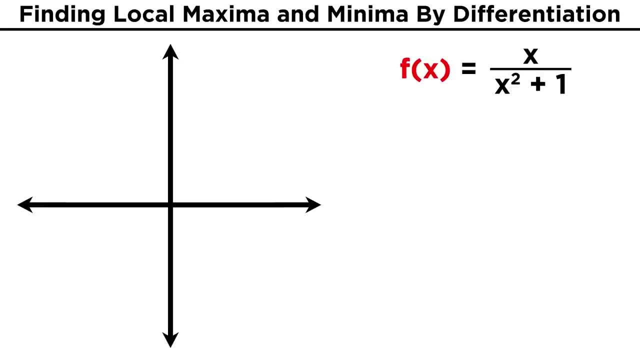 That one was pretty simple: quantity x squared plus one. Again we must take the derivative and for that we need the quotient rule. Remember it's bottom times, the derivative of the top minus top times the derivative of the bottom over bottom squared. 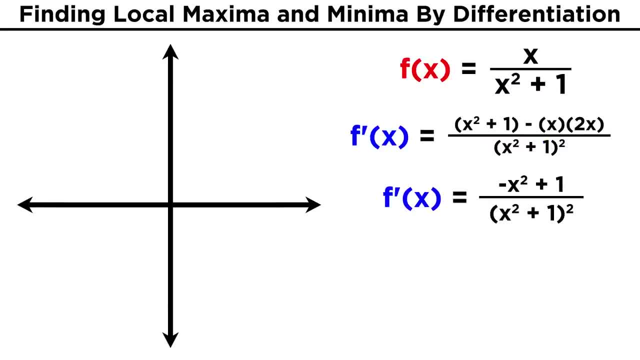 Here. that gives us this, and we can simplify to get negative x squared plus one on top. Now remember to find the zeros of a rational function like this one. we just need to find the zeros of the numerator, since zero over anything is zero. 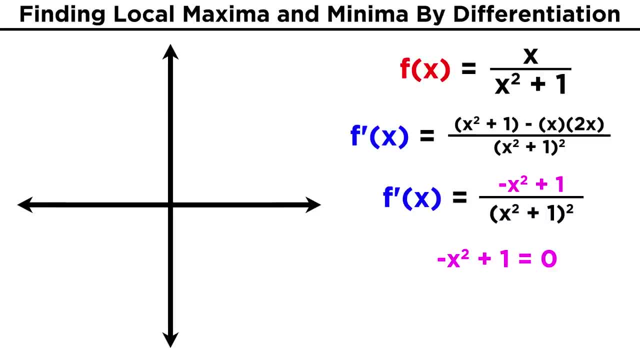 So let's set negative x squared plus one equal to zero. We rearrange to get x squared equals one. take the square root of both sides and x must be equal to plus or minus one. That means that x equals negative one and one will give local maxima or minima on the 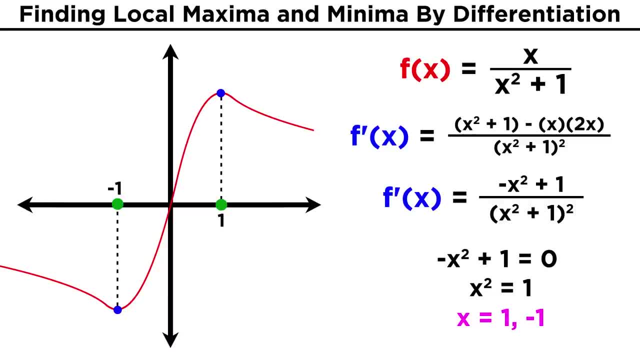 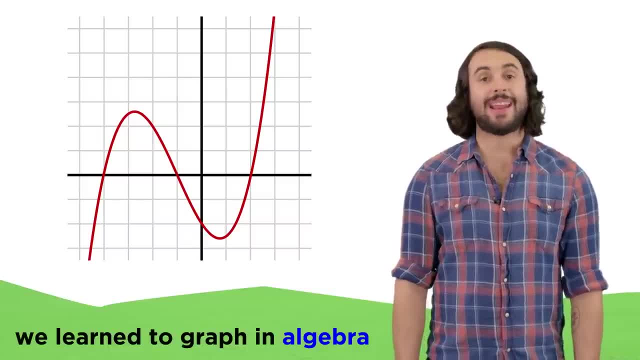 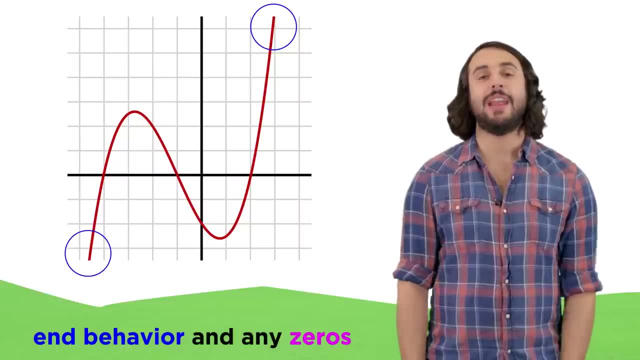 function, And in fact that's what we want. The function looks like this, So this is one great application of differentiation. In algebra, we learned how to get a rough sketch of a higher degree polynomial by finding the end behavior and its zeros, but it was always a pretty rough sketch, as we never